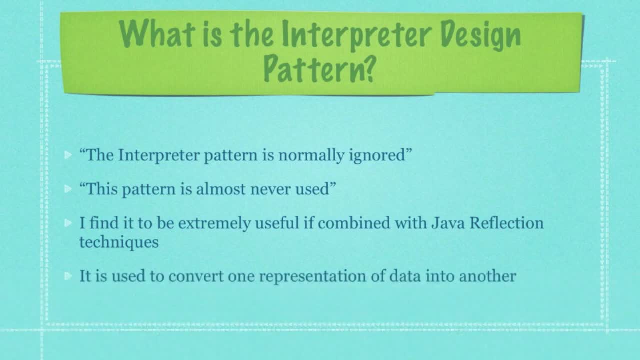 video right now and stop watching it. Also, if you are here for just a complete copy of the Gang of Four book and their interpretation of the interpreter design pattern, while I will, for the most part, stick to that, I am going to make changes. 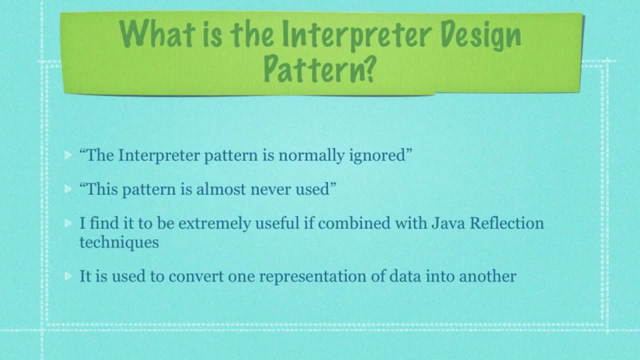 So if you don't like that fact, also go watch somebody else's video. If you do, however, want to see how to do some really cool things with the interpreter design pattern, you're in the right place, And let me just show you what we're. 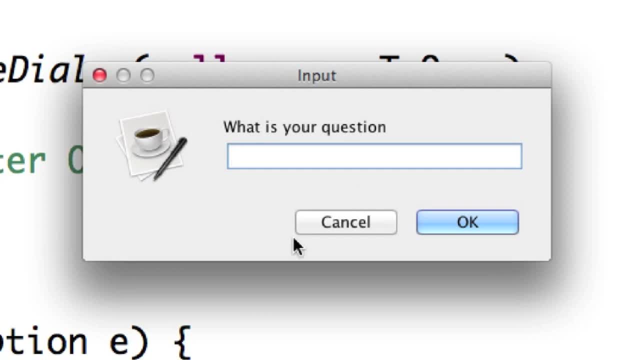 going to do So. let's say you would want to make a conversion little tool here so that you could convert different types of measurements to other types of measurements. Well, the interpreter design pattern is going to help you do that really easily. Let's say you wanted to. 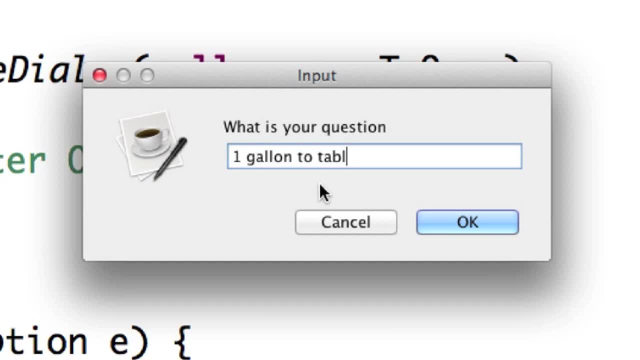 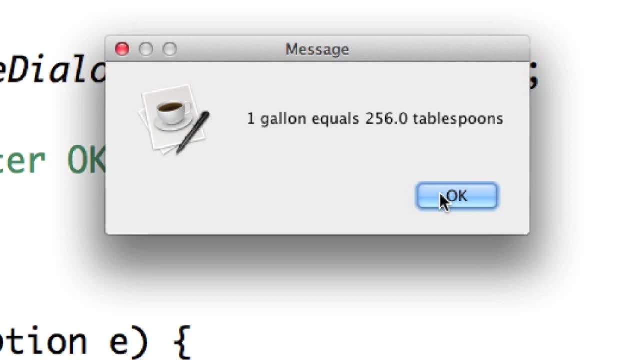 take one gallon and you wanted to convert it to tablespoons, That's all you need to do and hit OK and there's your answer. One gallon equals 256 tablespoons, And I could go in and type in all types of other different types of measurements, Like I mentioned before the previous professor who had talked about. 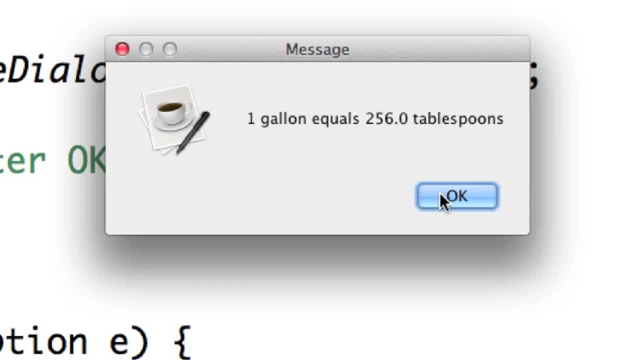 the interpreter design pattern pretty much said it was worthless That night, whenever I used it in combination with Java reflection, I was able to create. just with those two ideas, I was able to put together the Zork text-based video game. So if you want to see some really cool, 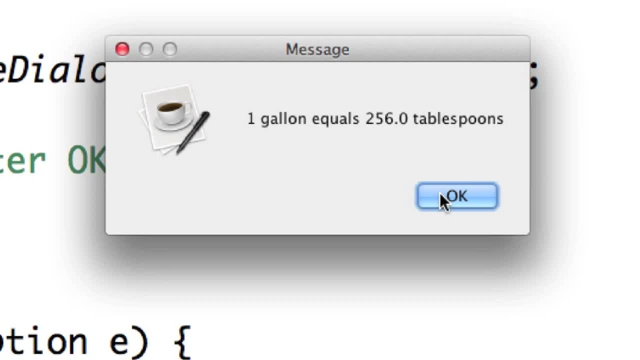 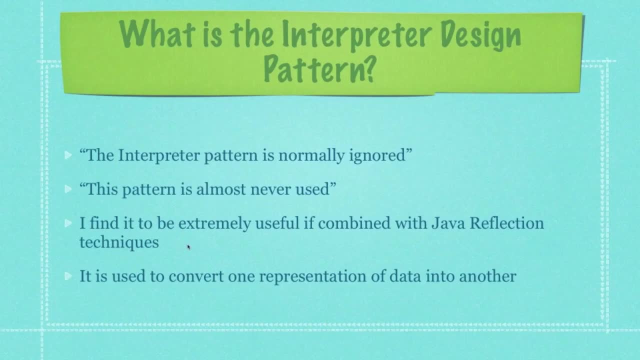 stuff and learn a whole bunch about Java reflection and a whole bunch of other things that I've received. in regards to questions you guys have asked let's get into the interpreter design pattern. So, like I said before, I find it extremely useful if used in connection with Java reflection techniques and pretty useful. 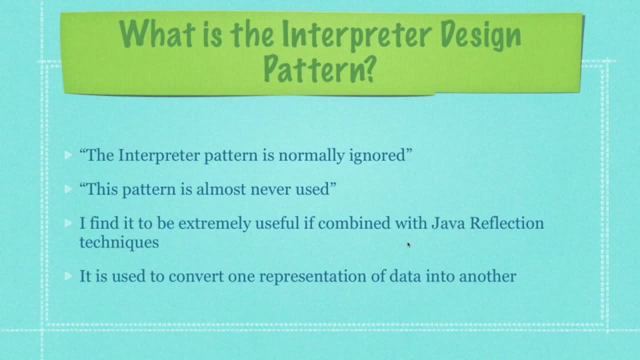 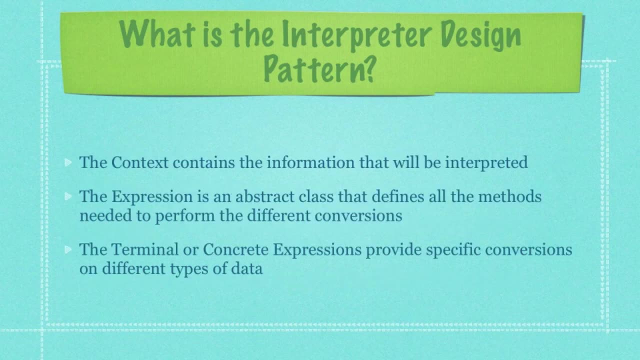 in general, It is basically just used to convert one representation of data into another representation of data. What you're going to have is mainly three pieces, and this all comes from the Gang of Four book. to a certain extent, You have the context, which contains all the information that is going to be interpreted. You have the 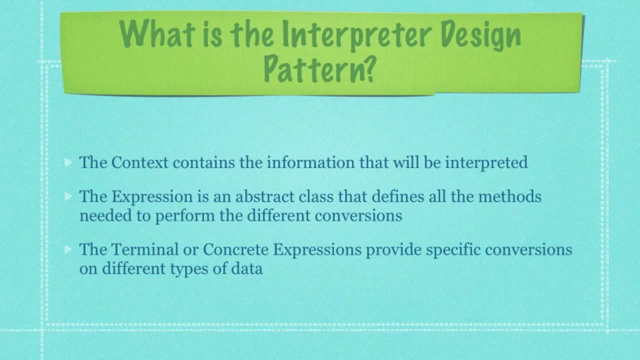 expression, which is going to be an abstract class that's going to define all the methods needed to perform the different types of conversions, And then you're going to have the terminal or concrete expressions, which are going to provide very specific conversions on different types of data. 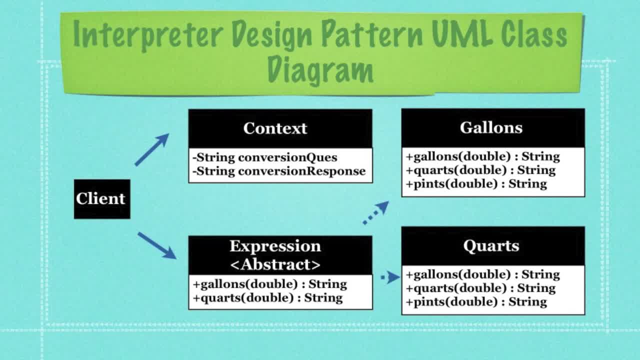 So let's look at this in sort of a UML class diagram. Okay, on the left you're going to have your client that's going to ask for certain information. That information is going to be stored in what is called the context And you can. 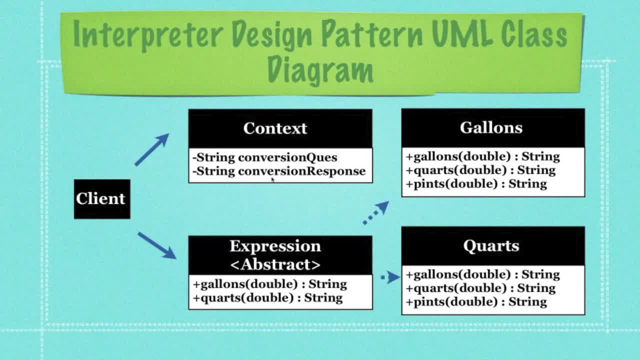 see that right here: conversion question. Then you're going to have all sorts of responses and different information is going to be relayed from the context over to concrete expressions that are all going to extend this abstract class, And you can see a very specific example. What I'm going to do here is I'm going to 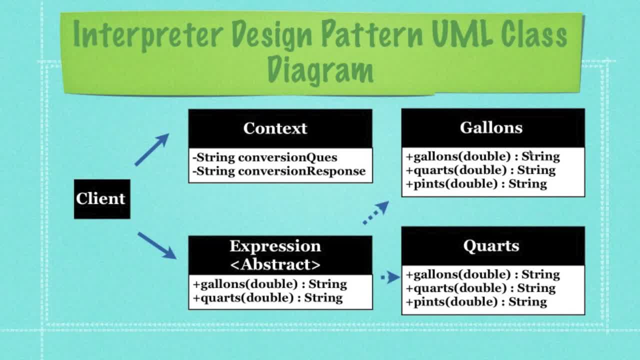 say: okay, you're going to give me gallons In exchange, I'm going to give you either gallons, quarts or pints. Or if you give me quarts, I'm going to give you gallons, quarts or pints as a response. So that's the basic idea of how the 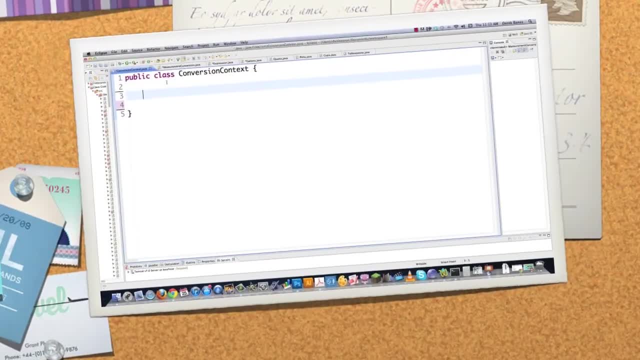 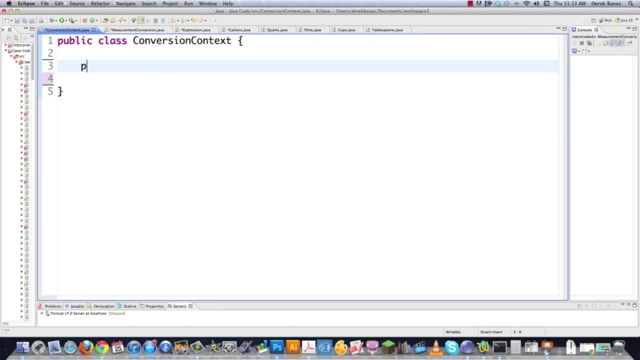 interpreter design pattern works, So let's jump into the code. Okay, so here I am in the conversion, or the context. I call this conversion context dot Java And I'm going to define a whole bunch of different things inside of here. So 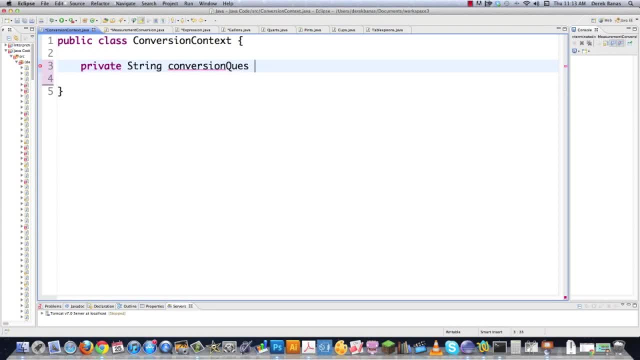 string conversion question is going to be the question gonna send, like I showed you in the example, which is, you know, one gallon to whatever you want to convert it to, And all the code is available underneath this video. It is heavily commented. if you have any questions, Of course you can. 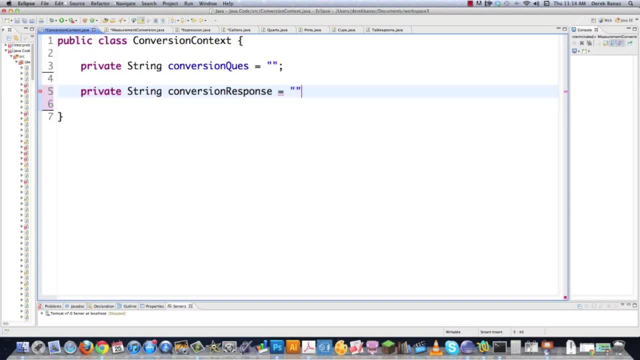 always leave questions down below. Then I'm gonna have conversion response And then I've also found the need to store from conversion, which would be something like gallons, which is what I'm going to be converting from, And then I'm also going to just store inside of here a string which is gonna be to conversion. 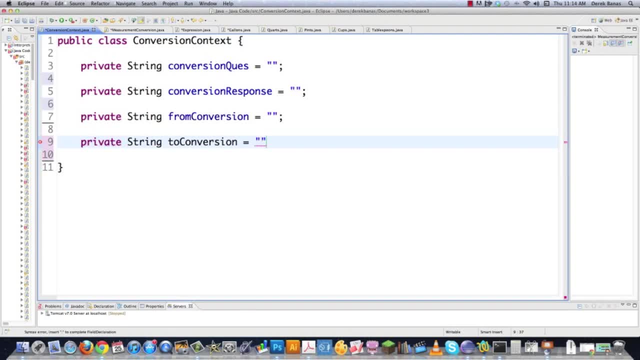 Which is going to be what I want to convert to. so let's say tablespoons or pints or whatever you want, And then I'm gonna create a string here, string array, and it's going to be Parts Meghan. It's gonna store everything in. 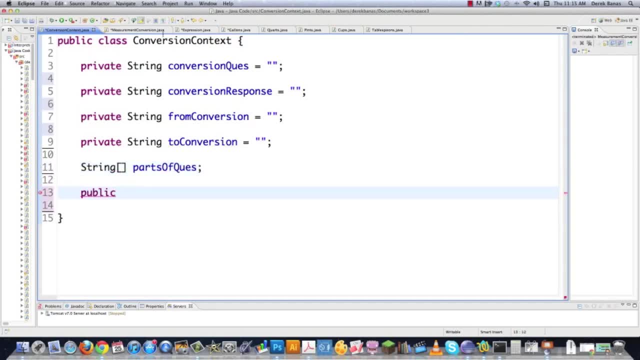 individual pieces. So then I need to create my constructor here And it's going to be past a string which is just going to be the input that is received from the user. Then I'm just going to go through there, I'm just going to go through here And then I'm just going to go through. 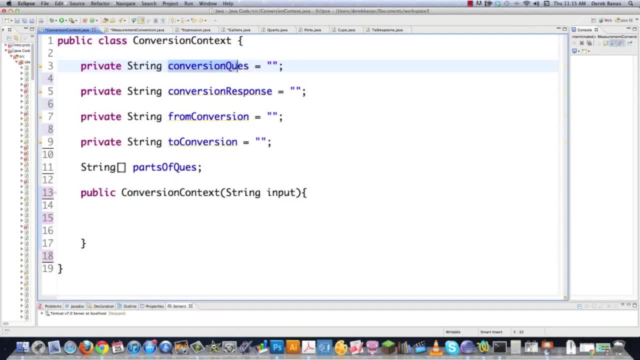 this. I actually don't have to do that. I can just do conversion. question is equal to whatever the input is. that's easy. then I'm going to go parts of question. I'm covering a lot of things I've received questions on in this tutorial also and I'm going to split that string into pieces based. 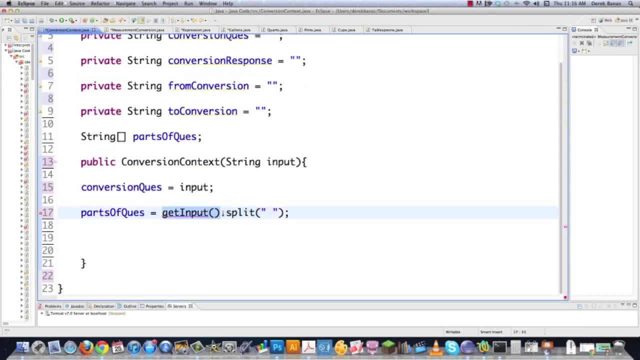 off of spaces and then get input. let's just copy that right there. I'm just going to create this so it's going to be public string, get input and it's just going to return conversion question, like that. so there, we got that all set up and then I need to get my from conversion and you can make this. 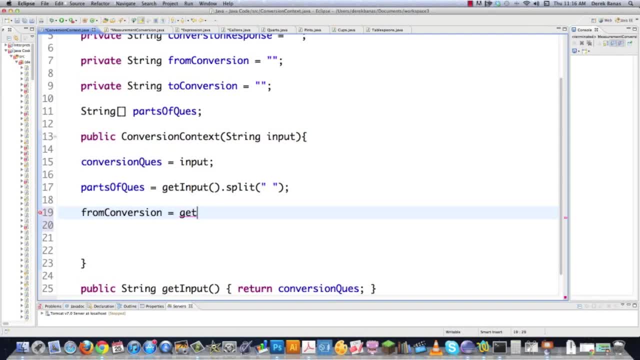 very, very sophisticated. like I said, I created a zork game from that which I was going to actually go over, but I just figured it would be way too long, so I'm going to try and simplify it, and then what I'm also going to do is capitalize this string so that it is easier to work with, no matter. 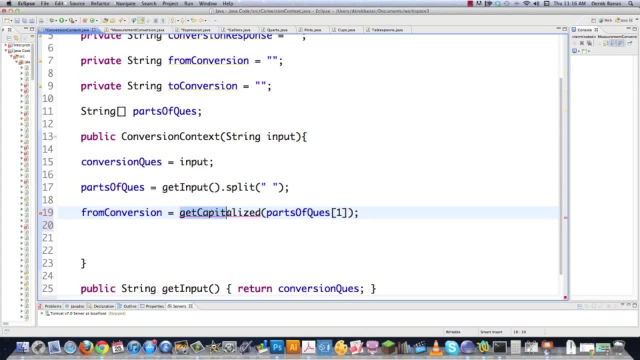 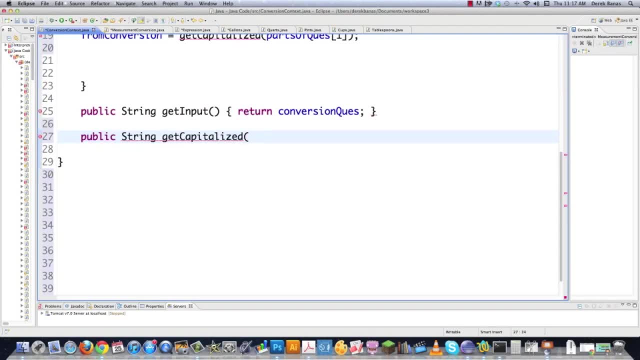 what sort of questions they ask. so that means I'm going to have to create: get capitalized. so let's bounce down here and go public string response: get actually. just paste that in there and it's going to get a string and I'm going to call it word to capitalize and the first thing I'm going 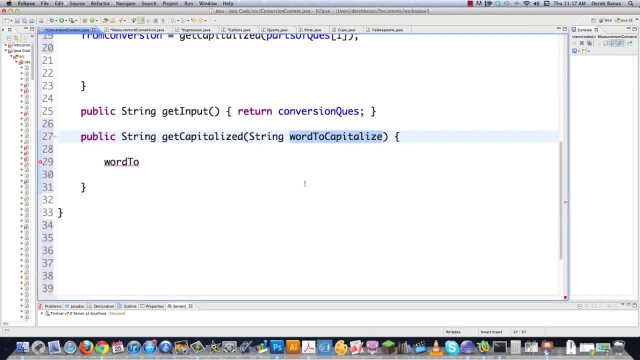 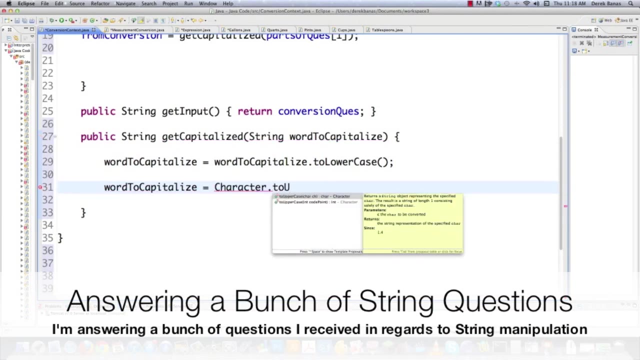 to do is actually put everything here that is sent to me in lowercase letters, and to do that just go word to capitalize and to lowercase, like that. and then I'm going to make the first letter uppercase. and how you do that is go character to upper case and I'm gonna go word to capitalize. 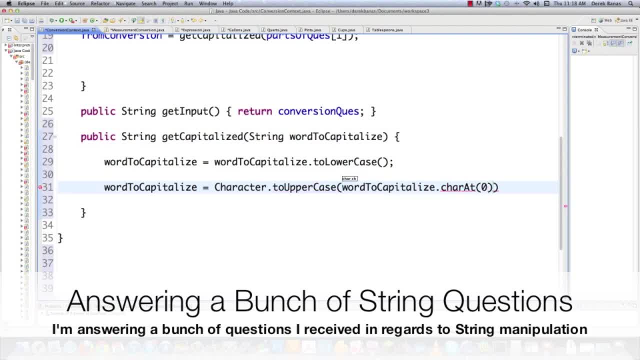 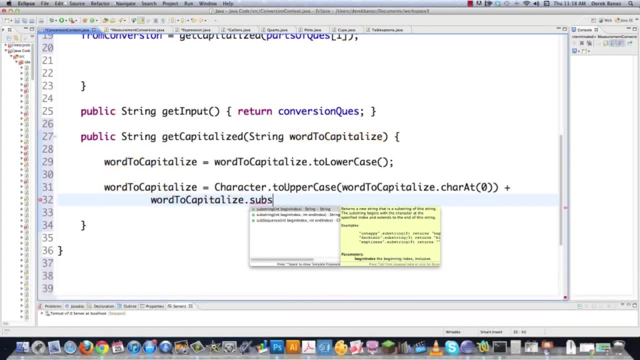 character at the zero index position, which is, you know, the first character in the string plus there, and then go word to capitalize and type in substring one like that, and that's going to capitalize just my first letter, and then on top of that I'm going to throw a couple other things. 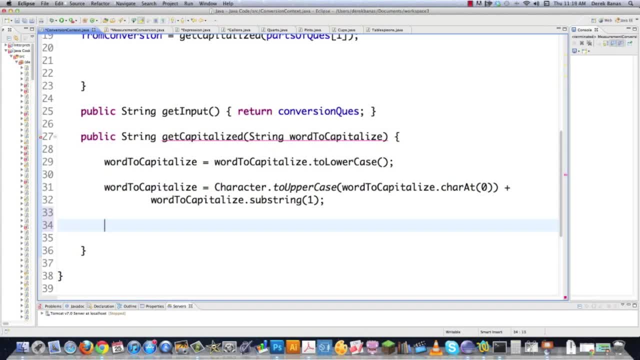 I'm gonna put an S on the end of this. so if they say one gallon, two pint, it's going to work, and if they say one gallons or two gallons, two pints, it's also going to work. so to do that, I'm going to go int. length of word is equal to word. to capitalize, I'm going to get the. 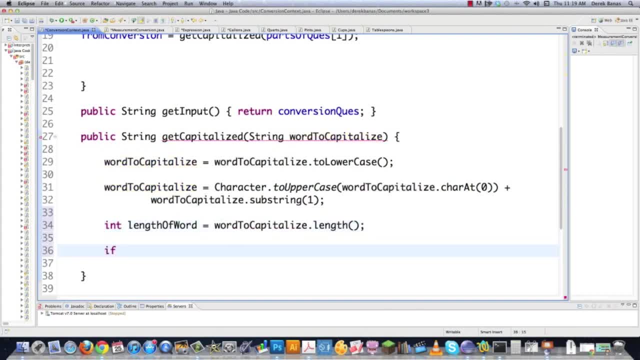 length of this. so that's, I'm going to get the length. then I'm going to say if word to capitalize dot character at, and I'm going to type in length of word minus one, which is going to get me the last character inside of this guy, and then after this I'm going to say is not equal to s? well then, 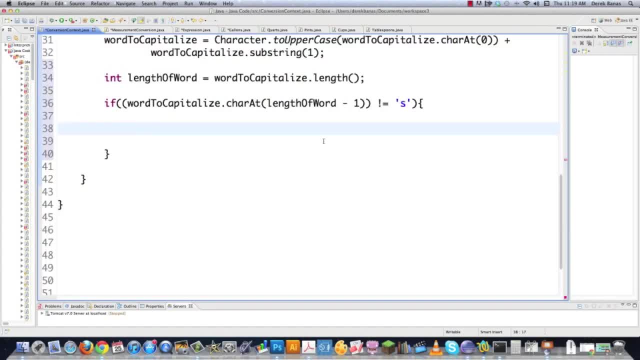 I want to put an s at the end of it so that we'll be able to once again to work with gallons or gallon. so we're going to go word to capitalize is equal to new and to insert a character into the end of the string. I'm going to use a string buffer and go word to capitalize and then after that, go. 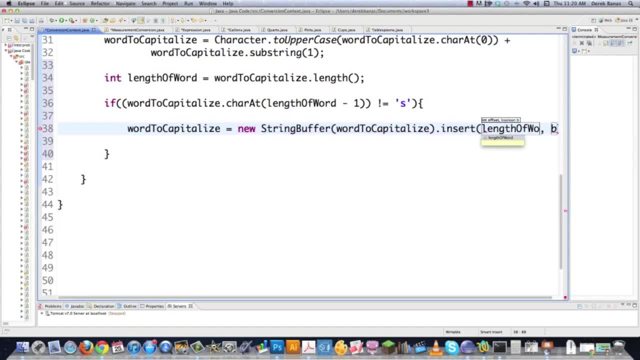 insert. and then we're going to say length of word comment there. and then I'm going to say that I want the index, the very last index in this string, to be changed to s, and then I have to call to string and then put that there. so that's going to insert the letter s at. 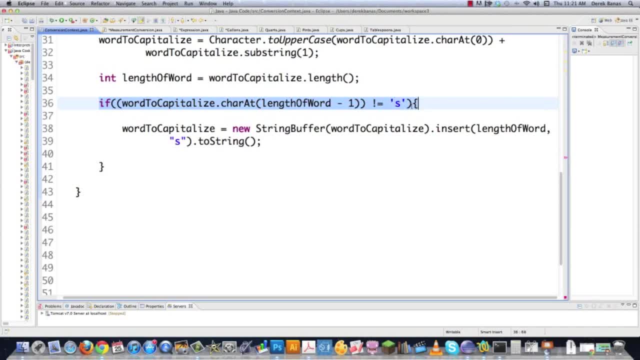 the end of the string if it doesn't exist, which we checked right there. so that's kind of neat. and then, after we've done all of that, we're going to go return word capitalize and there it is. it's all set up. there's a whole bunch of different things we just learned, so that's kind of cool. 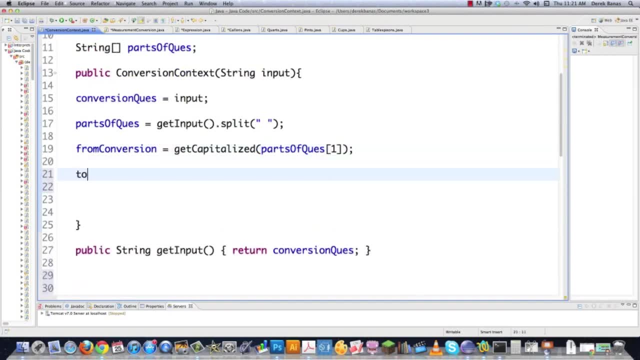 let's give myself some space. so there's get capitalized and then I'm going to do to conversion, which is going to be: what do we want to convert from two? so we want to go from gallons to pints? okay, well, that's what two conversions going to have inside of it. so we're 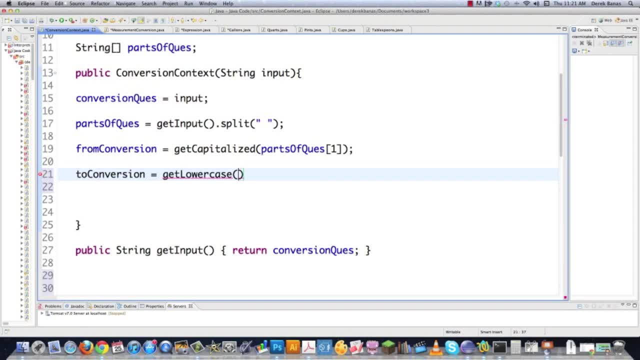 going to go get lower case and we're going to pass it hearts of, because I know what type string they're going to be sending me. we can change this to three like that, because I know what they're going to be sending me is going to be something to the extent of one gallons, two pints, okay, so 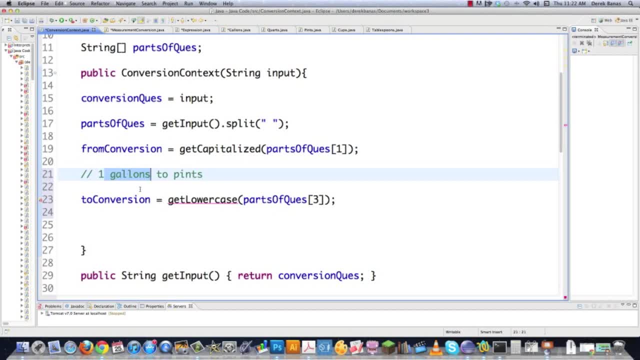 one is going to be this guy say gallons, right there, and then three, of course, is going to be zero. one, two, three, that right there. so that's going to be what I need to convert it to. okay, well, I'm using something else here. get lowercase, so I need to. 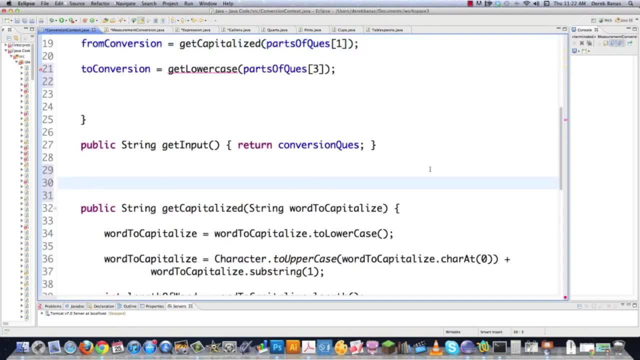 create that. let's just get that out of the way there and I'm just going to bounce right here and go public. I'm going to copy: get lowercase. it's going to return a string. get lowercase and it's going to receive a string and it's going to be word to lowercase. so we're just 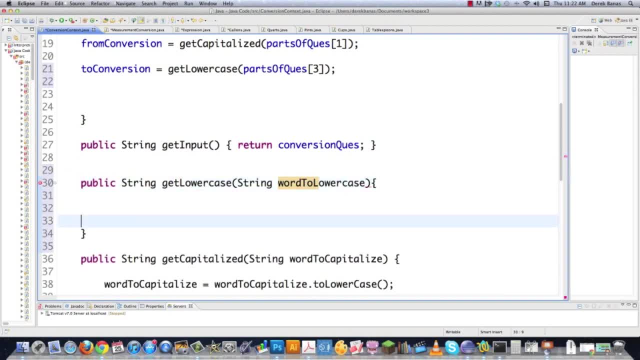 going to change this to lower case, like that, and then let's create our little method here and it's going to be real simple. I'm just going to go return word to lowercase and go to lower case, so pretty simple, and let's save that. so then we got that all set up, so then we're going to bounce up. 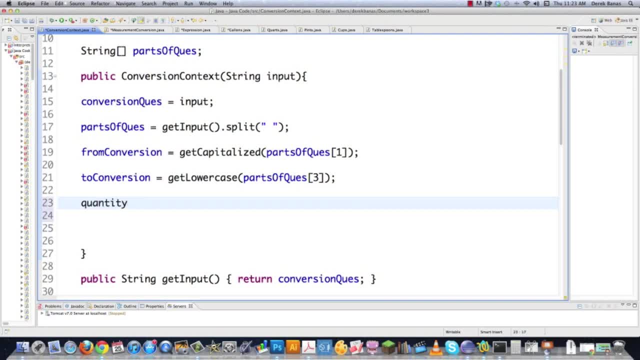 here again get some more information. we want to also get the quantity and we want to convert this into a double because it's a string right now. so we're going to go value of and then this is going to be parts of question, and the quantity is going to be the very first value passed. remember one: 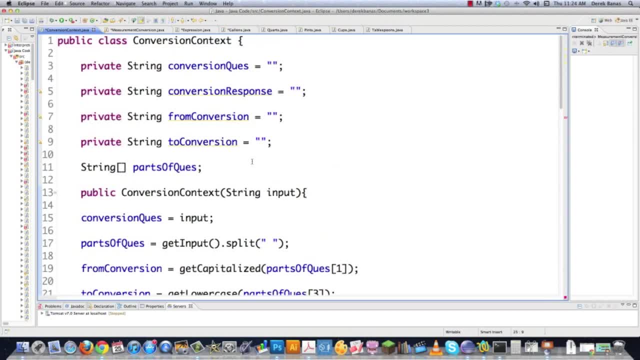 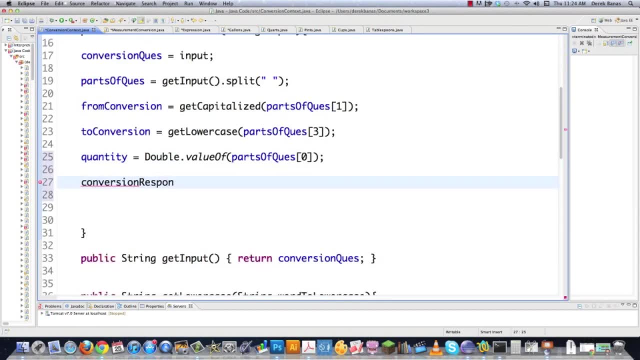 gallons, two pints. so the first index to be zero. And then I'm going to zoom up here and go double quantity, And then let's make this private as well, And then we're going to go: conversion response is equal to parts of question. 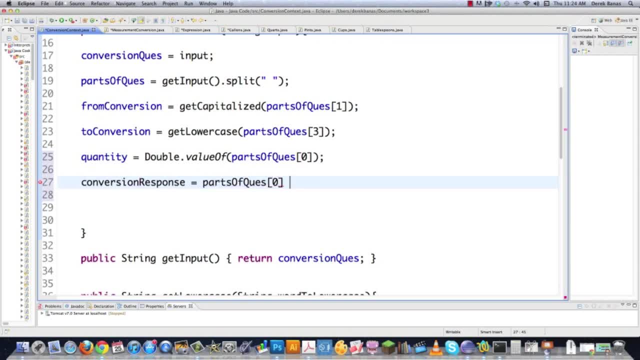 And I'm basically going to kick out the same thing. It's going to say whatever, like if we say one gallons, two pints, it's going to say one, throw space inside of there And then we can spit out either this or we could do that whatever, Let's just throw that in there. So that's going. 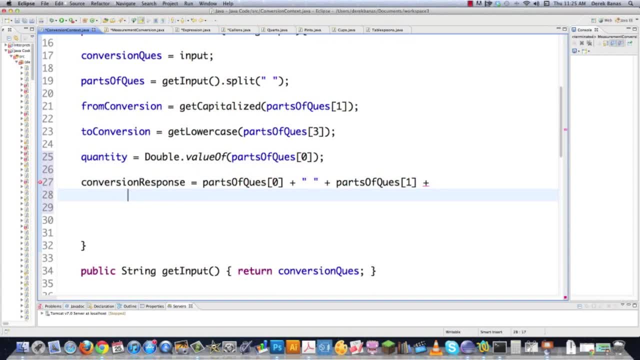 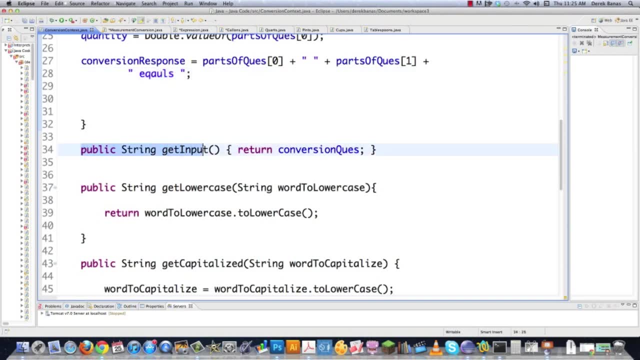 to be one gallons And then after this we're going to go equals And then later on we're going to put the rest of our conversion information in there. So then we need to output and return some different information in regards to, let's say, we want to give them the from conversion. Well, get, 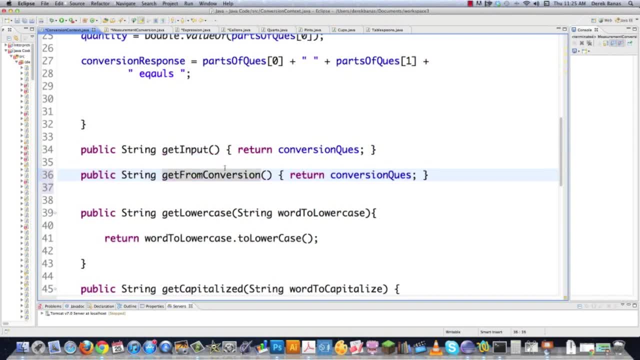 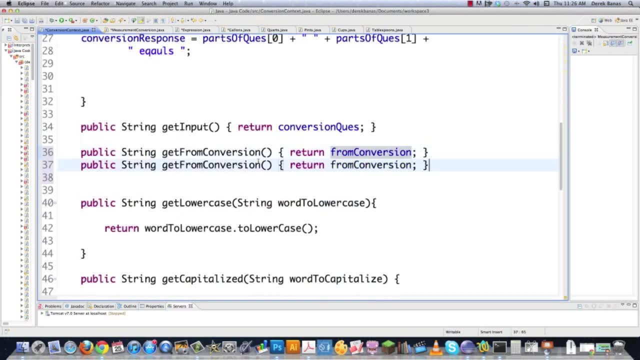 and I'm just going to change this to from conversion And it's just going to return from conversion, which is going to be right here. copy that, bounce down, paste that there And then we're also going to return to conversion. So there's two conversion and then we're just going to return to conversion And 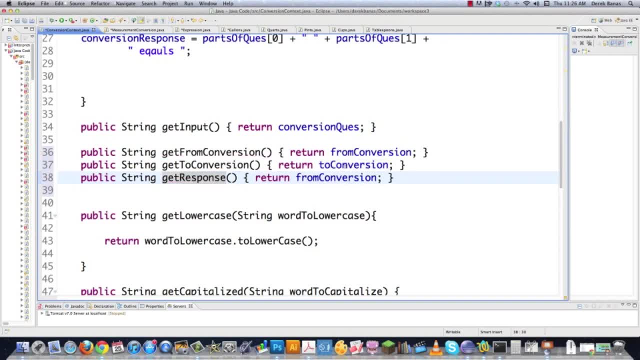 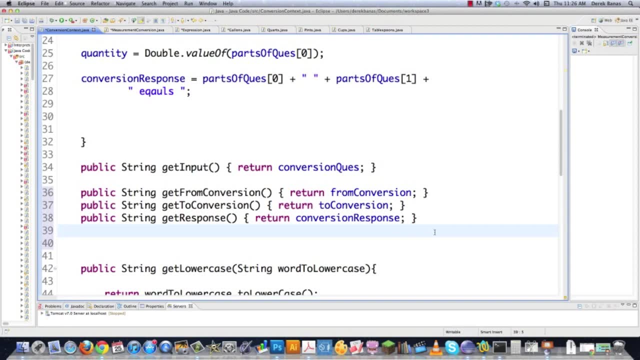 then we could also return get response maybe, And then this is going to return conversion response, which is right there. If you haven't been able to figure it out yet, there's a whole bunch of things being covered in this tutorial, aside from just the basic pattern. I could 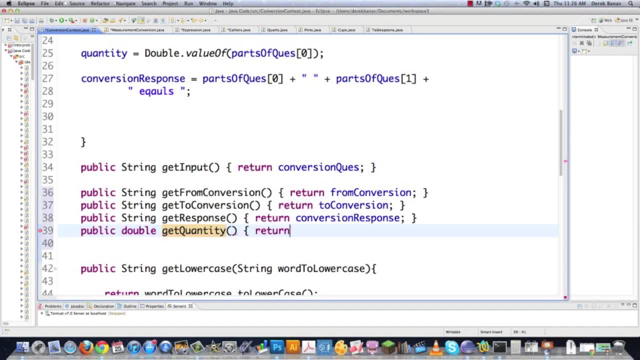 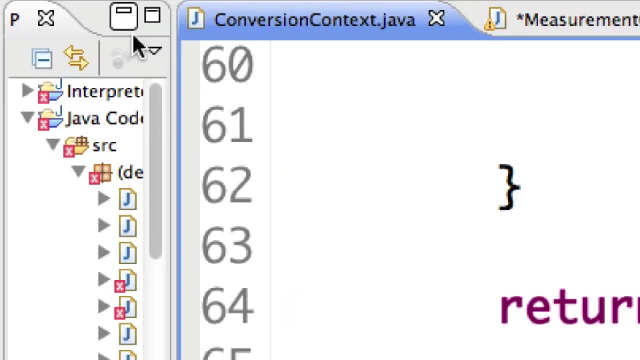 definitely see why we're going to need to get the quantity. So let's just return the quantity And that's all we're going to need. So there we are. we're going to file save that And that is conversion. Context dot Java that we got set up there. So the next thing we want to do is go into expression dot. 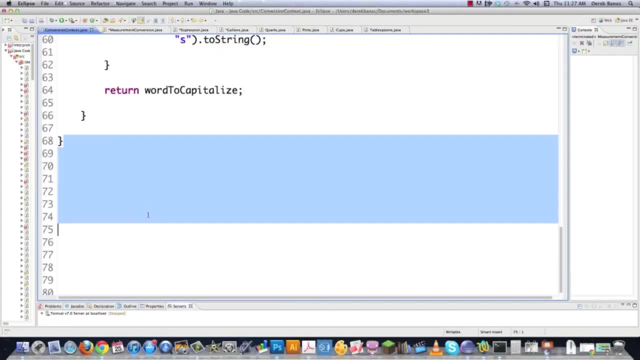 Java and define all the different methods or things that we're going to be converting into. So here's expression dot Java And, like I said, it's an abstract class And you can make this list a mile long and be able to convert into just about anything. So we're going to go string. Now let's 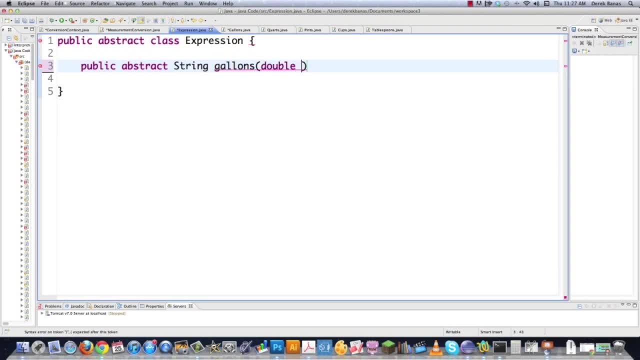 say, I want to be able to convert two gallons, So we're just going to go double and it's going to receive a quantity, So we got that all set. Then we have to think about all the other different things that we might want to convert to. So we 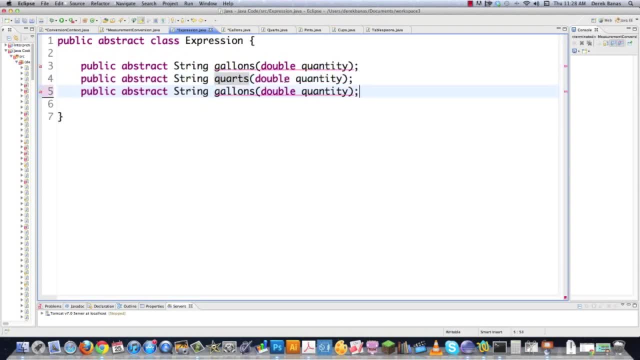 might also want to convert to quarts. So there's quarts. We also might want to convert to pints. So there's pints. We might also want to convert to cups, And then finally, let's convert to tablespoons. And there we are, We're done with that. So that is the expression. You're basically. 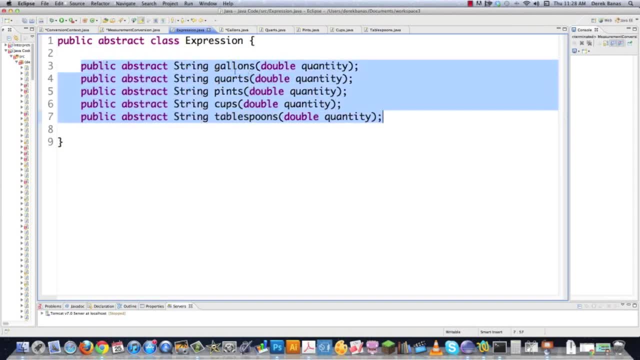 going to define all of the things that the concrete expressions are going to be able to convert into, which would be gallons, quarts, pints, cups and tablespoons. Like I said, this could be a mile long and be able to do really insanely awesome things. So now we're going to implement. 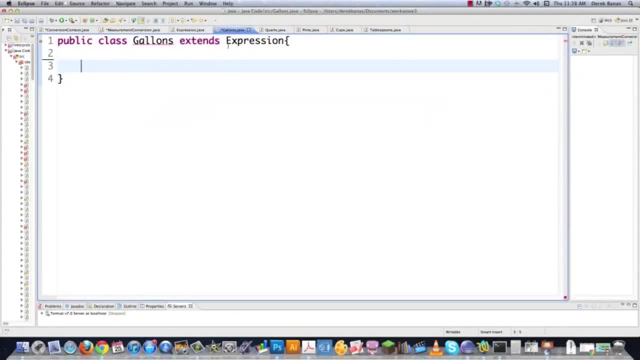 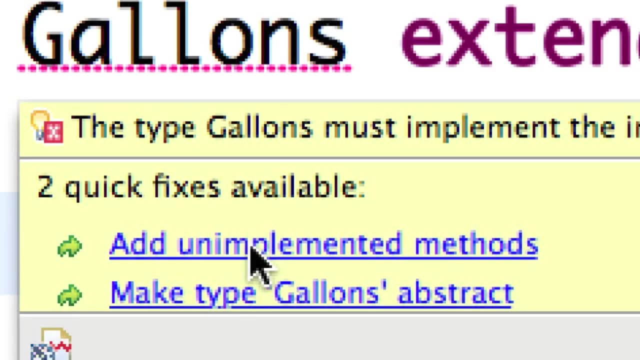 that inside of gallons dot java, You can see here Public class gallons extends expression. We're going to go here, zoom in on this and it's going to say, hey, you need to implement some methods. OK, fine, Do that for me, because I'm lazy. And there we are. Now we got all. 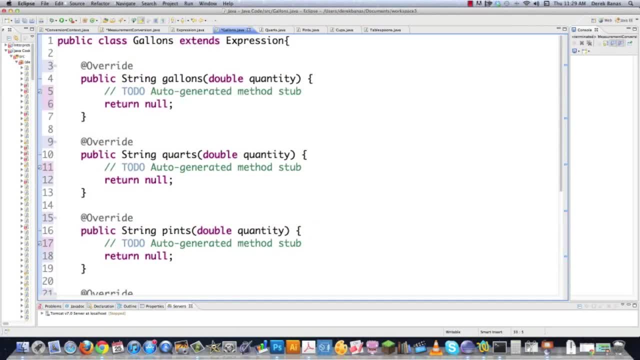 our methods we need. So, basically, if we're going to be converting into gallons, what do we need to return? Well, gallons into gallons is equal to gallons, So we're just going to return whatever quantity they send to us. So that's really easy. However, we're going to want to convert 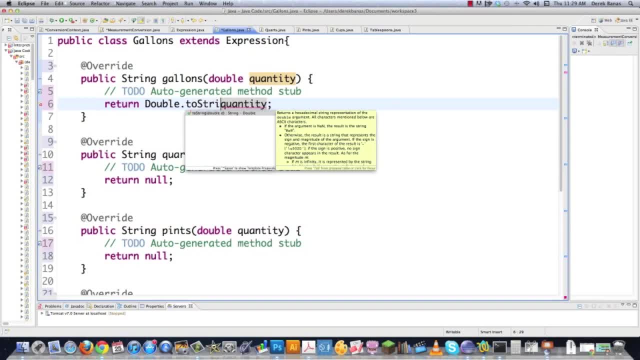 this into a string. so we're going to go double to string like that and then close that off, so that's going to convert that double, that's sent over into a string and then we're going to basically have to do that for everything else that we have here. let's just get rid of all those paste. 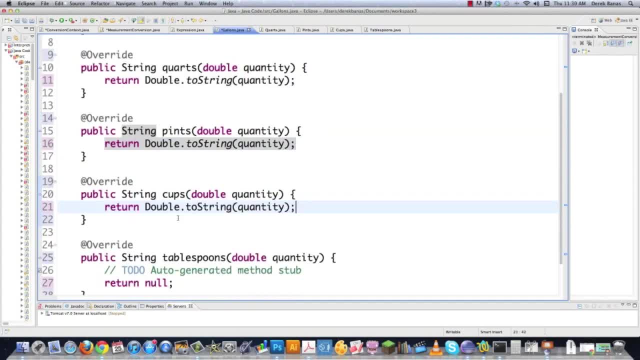 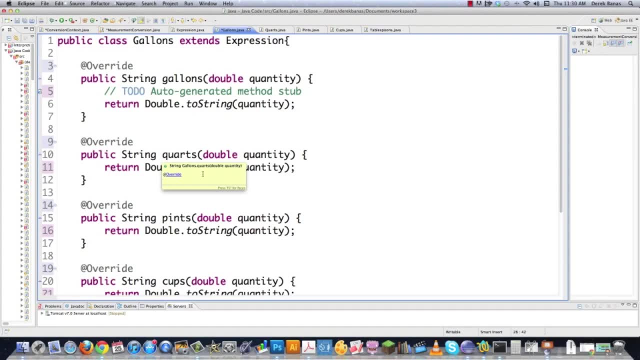 that in there, and then it's just a matter of doing the conversion, which is about math and it's not really about programming. but either way, let's do it right. so how many gallons goes into quarts? well, basically, you're just going to come in here and multiply quantity times four. here, for pints, we're. 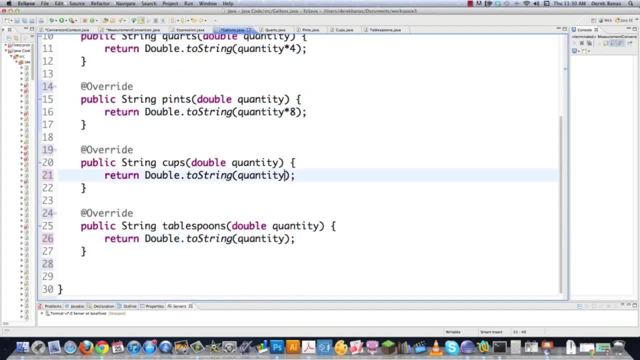 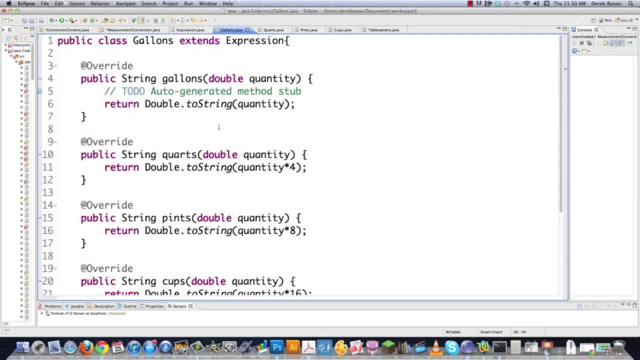 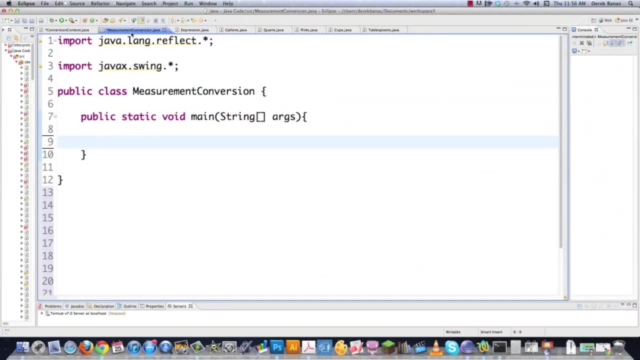 going to multiply this times eight. and then, for cups, we're going to multiply that times 16. and then tablespoons, we're going to multiply that times 256. and there you go. we've just defined our conversions. so we're done. I'll save. okay, so now that that's all out of the way, let's go into. 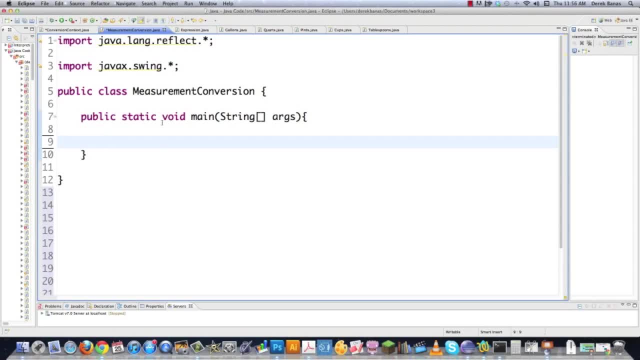 measurement conversion dot java and let's start playing around with reflection. as you can see, here is the library and we're going to use a couple little swing tools just to help us along so that we have our little pop-up that shows on the screen. so the first thing we're going to do is we're going to go. 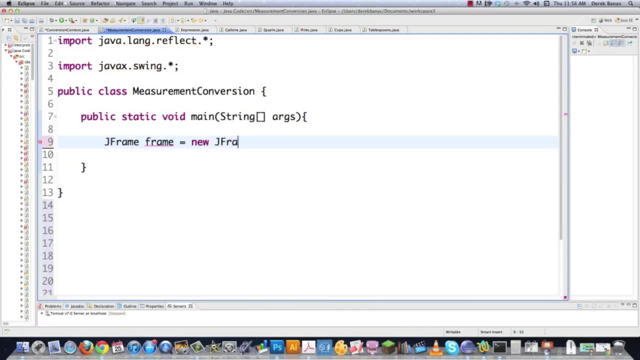 j frame frame is equal to new j frame so that we can open our little pop-up on our screen and then we're going to go string question ask is equal to j option pain, which is our little pop-up whenever we put in show input dialogue and then we just need to pass it the frame that we want to use. 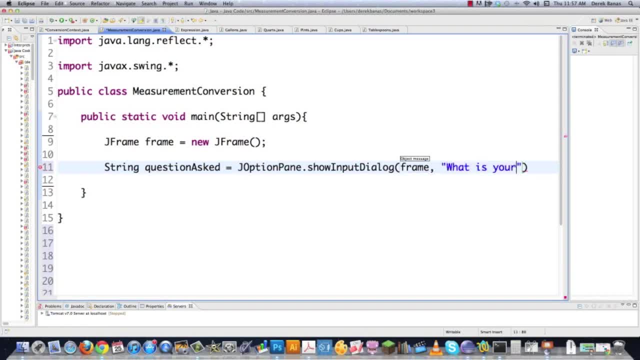 and the question we want to ask is the same thing we're going to do is we're going to go ask which is what is your question? and there we go. now we're going to get our string, which is going to contain the question, and it's going to be up to us to be able to translate this into an answer. so 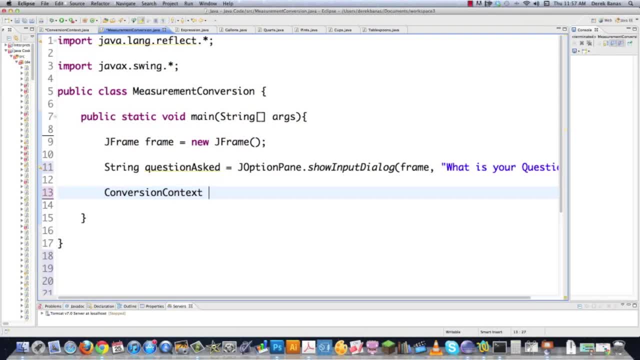 then we're going to go conversion context, which is the very first class that we created and we're going to go question is equal to new conversion context, which is going to store remember the initial response or information that is sent to us and we're going to pass that question asked and 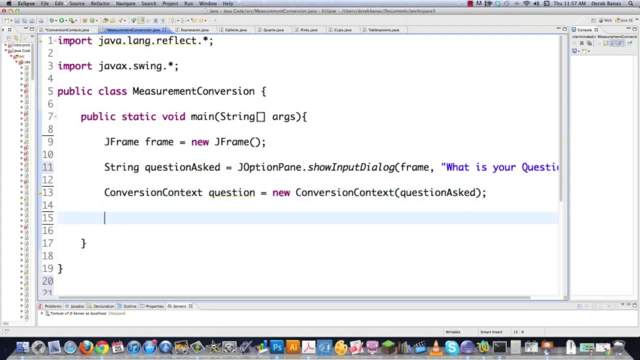 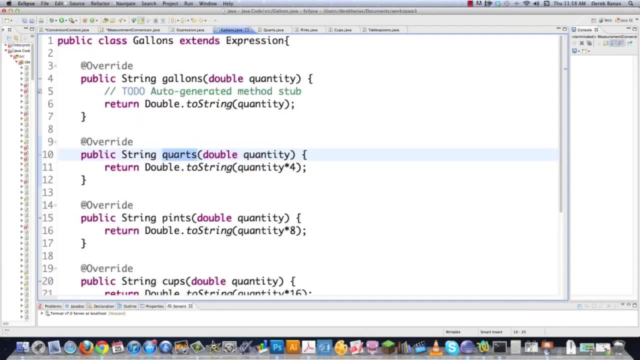 it's going to be it's job to parse it and put it into different forms that we're going to be able to use. well then we're going to go string from conversion, which is going to find the object class that we're going to be converting from see. in this situation, we're going to be converting from gallons to either. 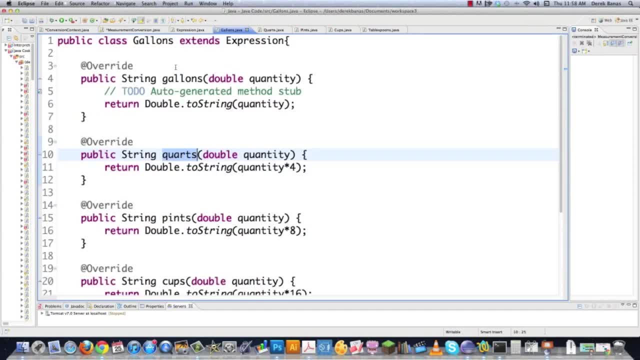 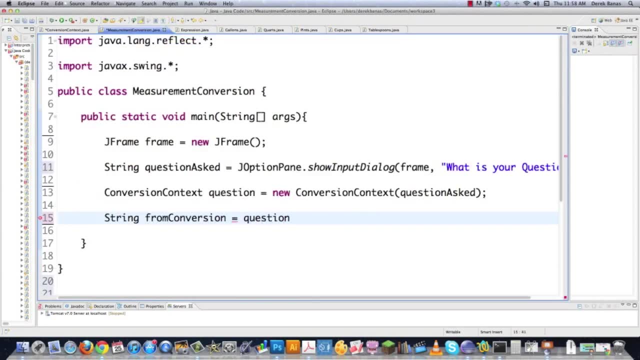 gallons, quarts, pints, cups or table spins. so from conversion means that we're referring to this class right here. so let's go into that and to get that we're just going to go question: get from conversion. we're going to call that method we created earlier and open that up. well then, we're going to need some other information. 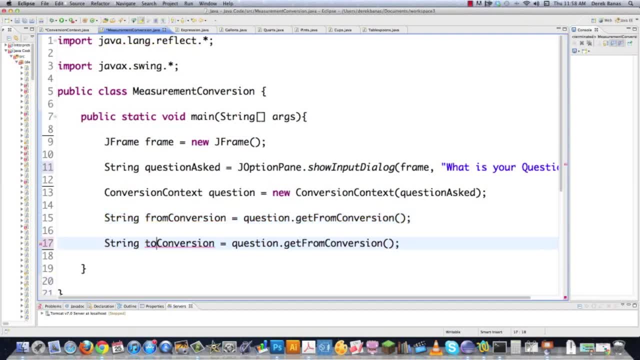 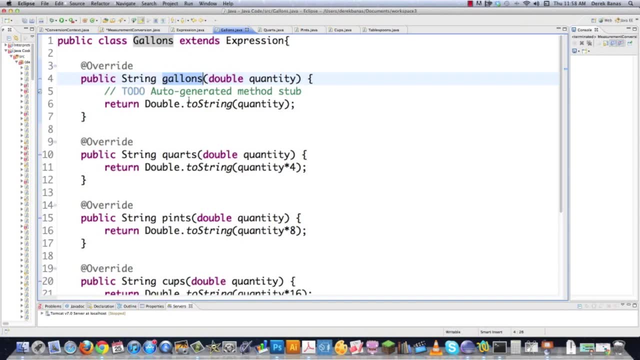 like: what are we going to be converting to, or the to conversion. now to conversion is going to be a reference to the method we're going to be calling. we're going to be using reflection again and i'll put a link to a reflection tutorial below if you don't know what that is, and there that. 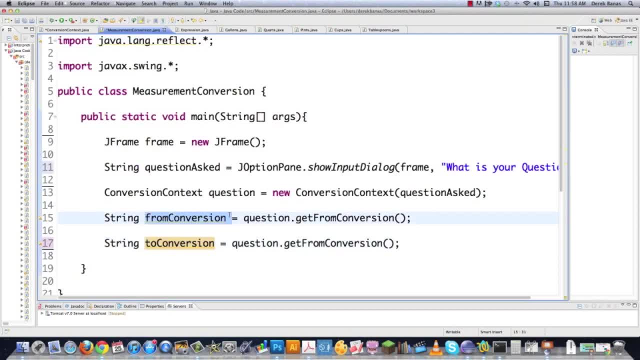 is. so that's going to be. this is going to be the class object we're going to be calling and this is going to be the method we're going to be calling within that class object. so get to conversion and, for the most part, like i said, that we're sticking to the basic gang of four. 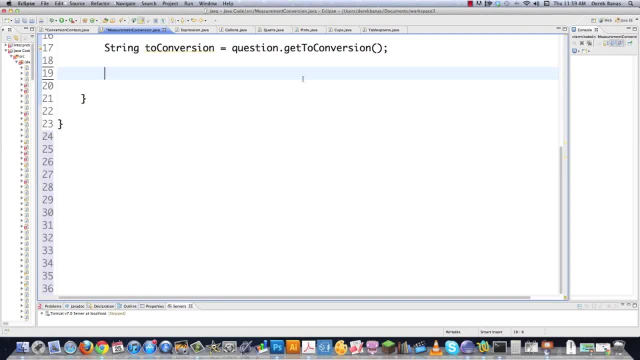 interpretation of the interpreter pattern. but i'm adding a whole bunch of other functionality to make this really cool. well then, we're going to go double quantity. we need to get our quantity that we are going to start with. so get quantity is going to do just that. give me that and then we 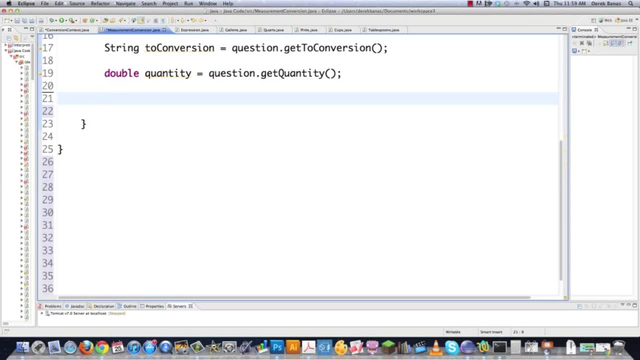 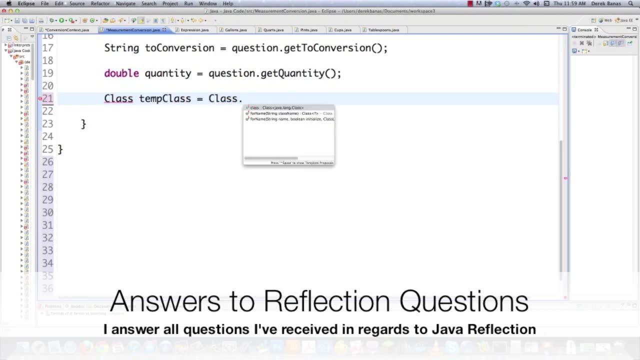 need to get the class based on the from conversion string or the class object. so how do we do that? we're going to go class, temp class and then we're going to use our conversion cool stuff for name, and if we want to call the class well, we just want to pass it from conversion, which. 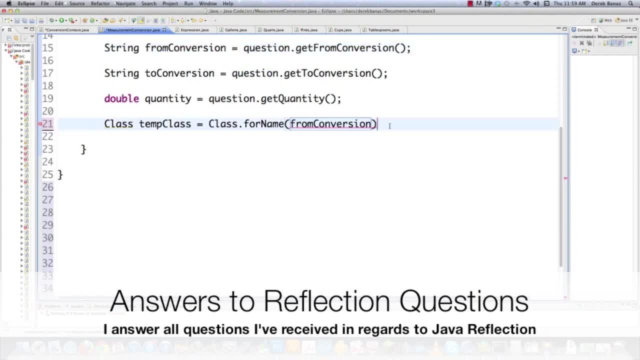 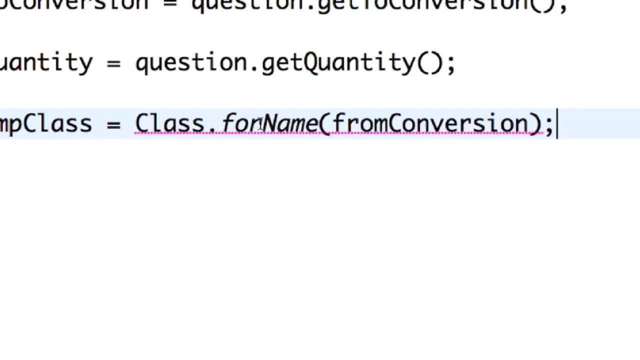 is going to be a reference to the class object that we are converting from, which is, in this situation, gallons, like i said before. so that's the class object we want to convert from, and it's going to give us some error message saying this needs to be surrounded with a try, catch block. 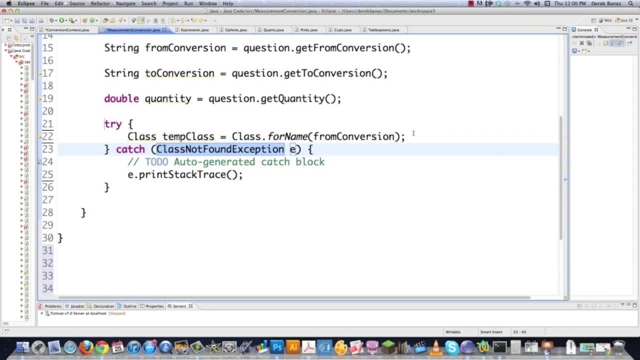 so let's just surround with the try catch block, let them do all the work for us, and then we're going to you, the constructor, dynamically for the conversion string and using reflection we're just going to go and create a constructor object and to call the constructor on our class we just go temp class. 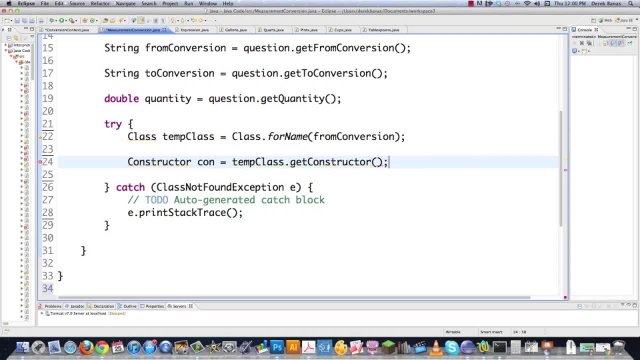 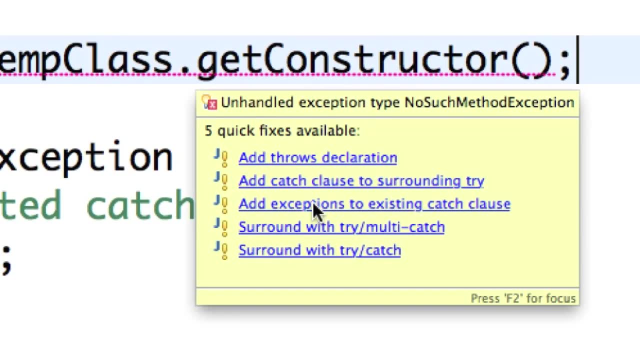 get constructor and it doesn't have any parameter types. so we can just leave it like that and it's going to give us another message that says, hey, we need to add some things to our try catch block. so let's just let it do that and just say: add catch clause to surrounding try keep everything. 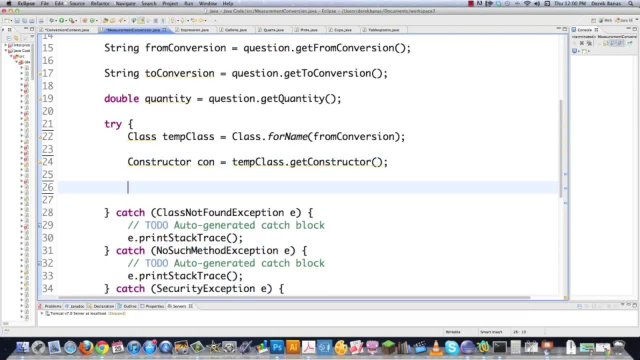 nice and tidy and it did that for us, so that's cool. now we need to create a new instance of the object that you want to convert from, and to do that you're going to go object convert from. and we know this is going to be an expression, because all of these extend the abstract class named. 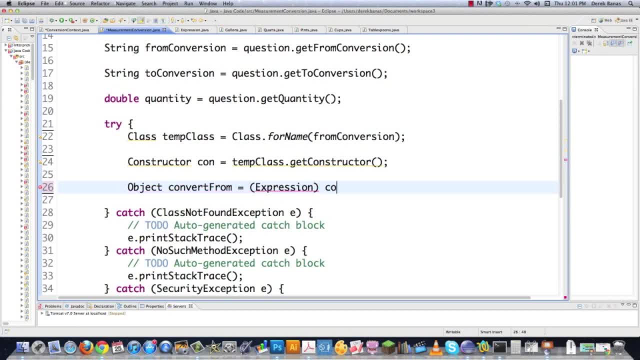 expression. so we want to tell it that, because that always is going to apply. then we're going to go con, which is a reference to the constructor, and go new instance and there are no arguments for the constructor, so we can just leave it that way. and what's it going to do? it's going to say: hey, 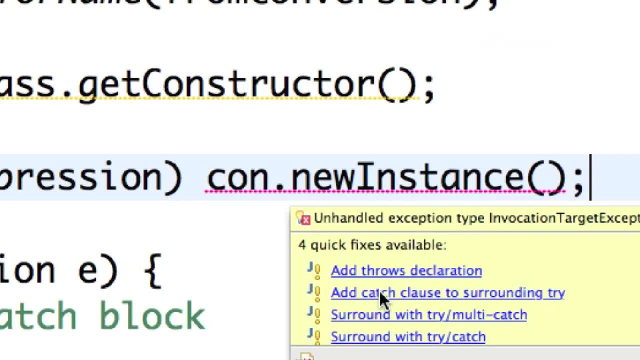 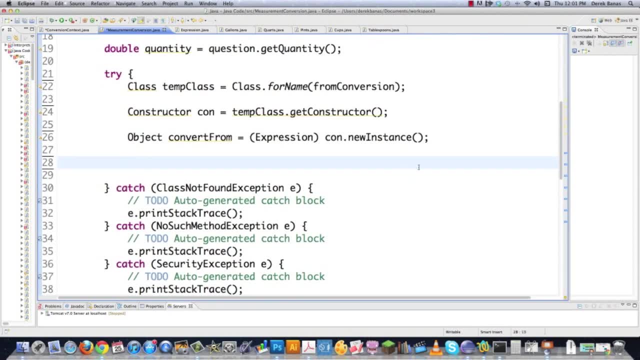 we need to add some more catches to our try catch block. add catch clause to surrounding try. click on that. we're going to do that again, so come back up here so we know what class we're going to be using, we know what constructor and we also created an object of that class type. so now, what are we? 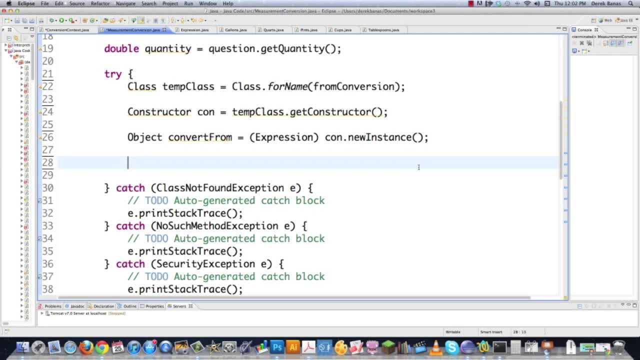 going to have to do is define the method parameters that are going to be expected by the method that was going to convert from the original chosen unit of measure to the new one. so let's just go over here. what is going to be sent to this? a double. that's all that's going to be sent to all of the 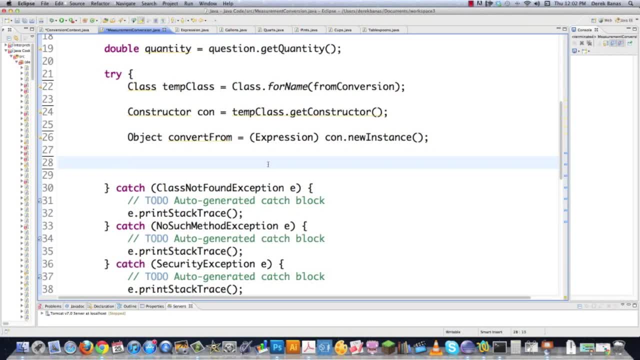 methods that we're going to be calling on. so we need to come in here and define that fact. to do that, we're going to go class, create a class, array, method parameters. we're going to go new class like this, and then we're going to pass it a double. so we need to go double type, and I talk about the. 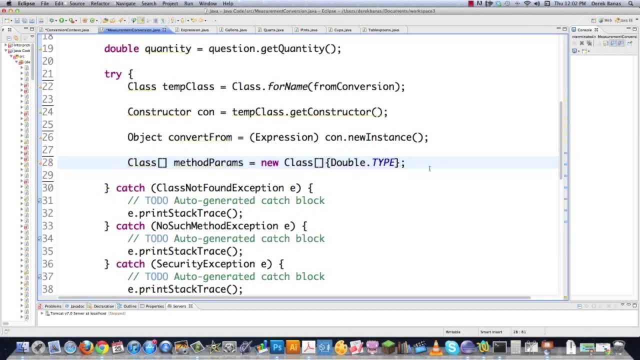 other types, but it's integer and all these other things. it's just basic common sense to figure out what type of class we're going to be passing. there's a double and that's what we're going to be passing. then we need to get the method dynamically. that will be needed to convert into our chosen unit. 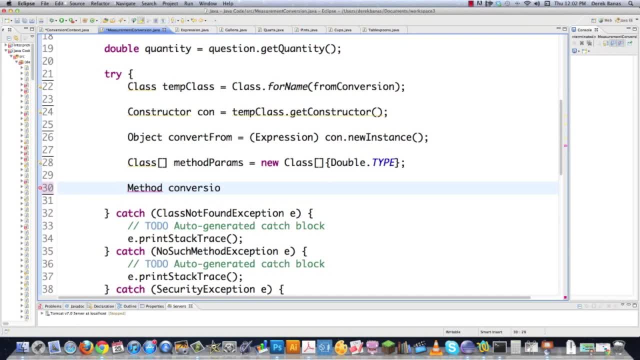 of energy. so we're going to go and create a method- object conversion method is going to be its name- and to get that we're going to go temp class get method, which is another reflection tool. and if we want to figure out what method we want to get, well, we 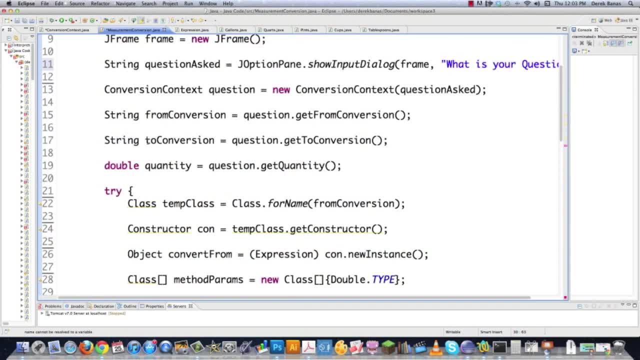 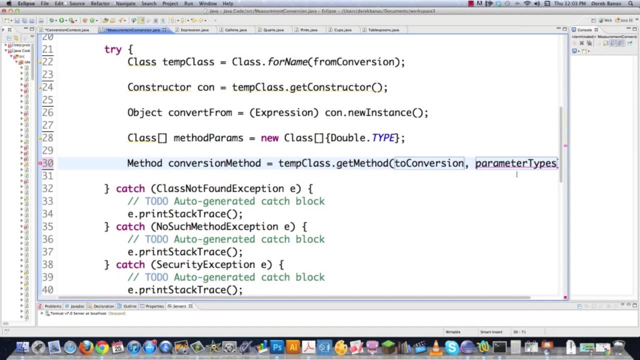 want to figure out. what do they want to convert into and to? conversion is a string that contains that name and that is what we're going to put inside of there. so there's two conversion and what's going to be passed to the method. well, this guy right here. so we're going to go method. 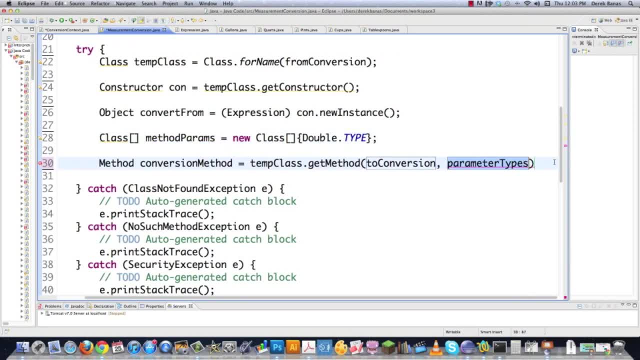 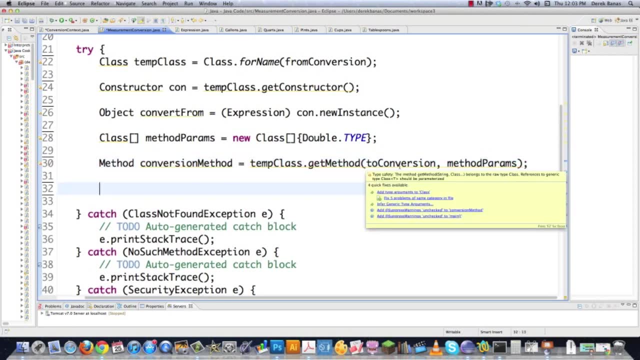 parameters and copy that guy and paste in method parameters. so this is what we're going to do. we're going to do is we're going to use the parameter type, which is going to be a double, which we defined above, and if you want, like I said, the codes underneath this video, well then we need. 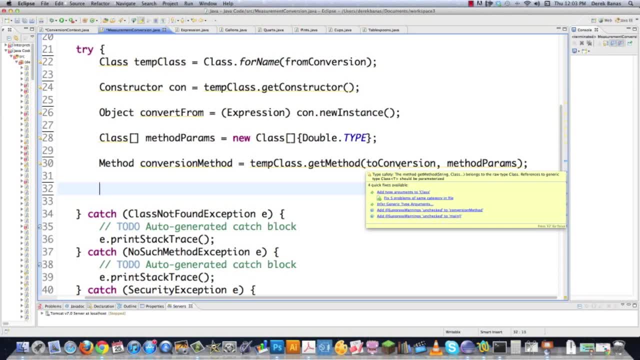 to define the method parameters that will be passed to this above method that we just got a hold of. and to do that, we're going to go: object and I'm just going to call this: params is equal to new object, and then we're going to pass it an actual double value. and what's a double value? 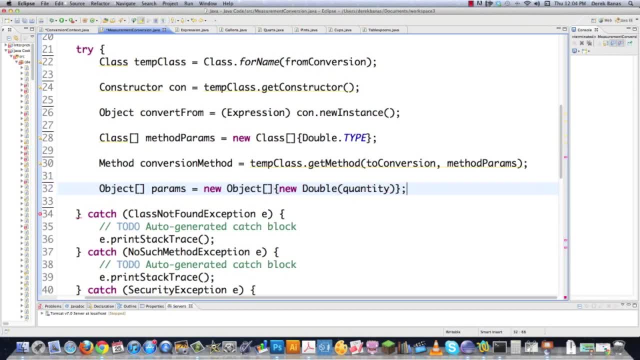 we're passing the quantity that is stored inside of here. so there we're actually passing a real, or there we're defining that we're going to pass a real double quantity or value over to our new method that we just created, and then we just have to get the quantity after the conversion, which is: 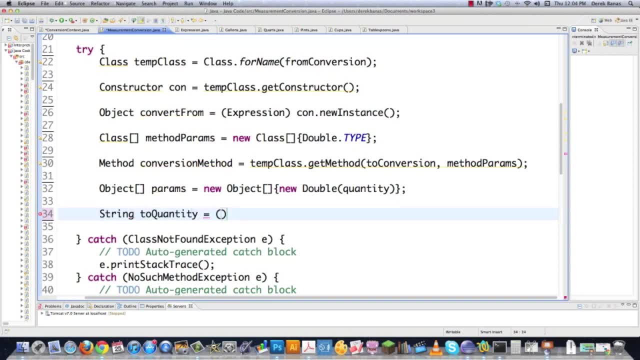 real simple. we're going to go string to quantity and then we're going to have to convert this into a string. so there's the cast conversion method. we're going to call that method. and how do we call method? using reflection, we use invoke, and then we're going to say, okay, well, what object? 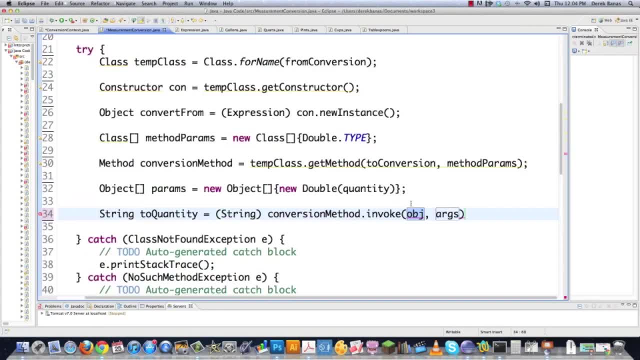 well the object's name, remember gallons. do we get this object? it's actually stored right here, see convert from. so we have to get the object that we're gonna be calling the method for and then, inside of that, we have to pass the actual values, or the double that we want. 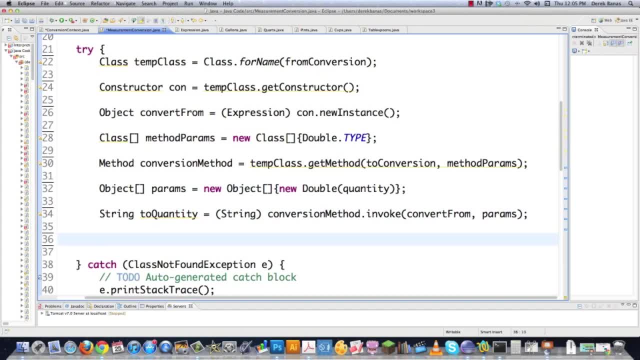 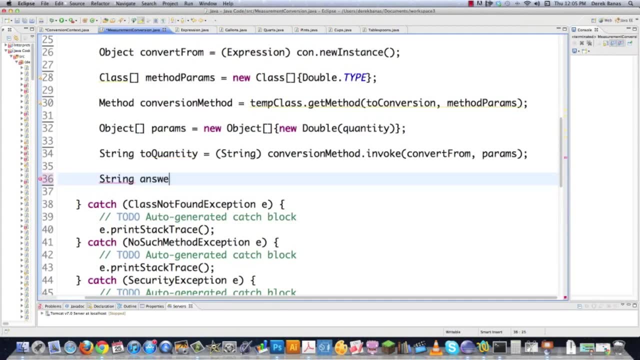 to pass to that very specific method. so this is powerful stuff. might be a little bit hard to wrap your head around sometimes, but it's really cool whenever you do. and then we're gonna go string and we're gonna go answer to question. we're done all the hard stuffs done. so if you have any trouble with any of this, 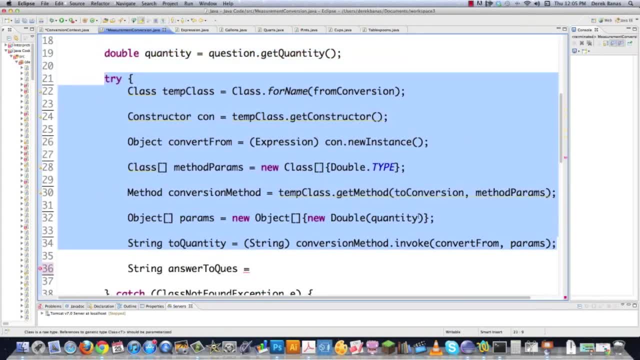 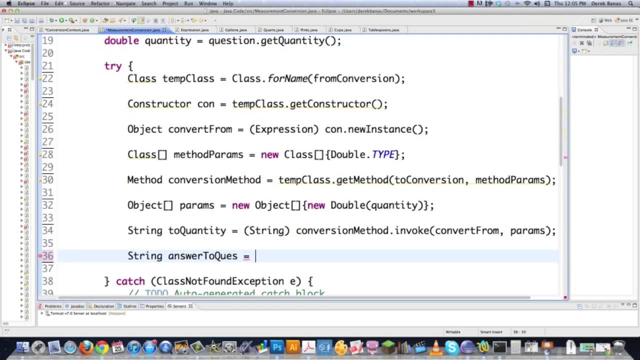 chances are, it's this stuff right here, and the only reason you're having trouble with it is you don't understand how reflection works. if you study this, you will you'll know everything you want to know about reflection. so then we need to craft our answer to the question, which is gonna be pretty simple. we're 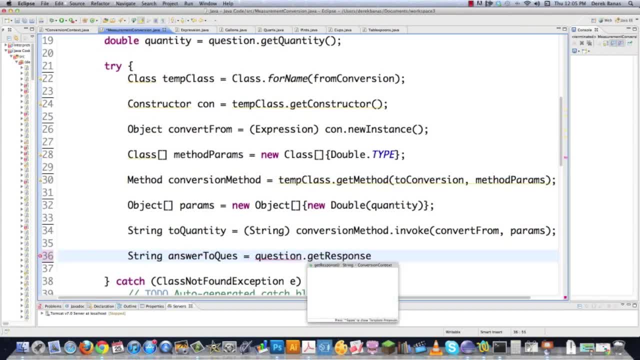 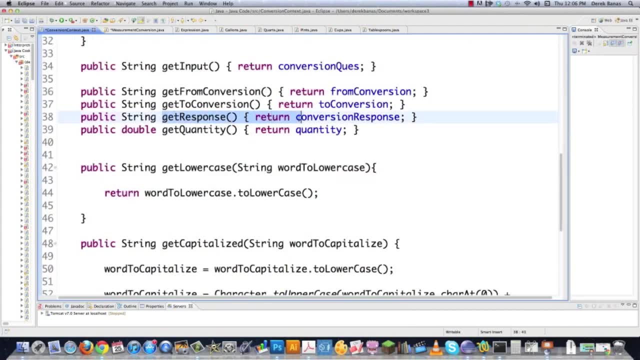 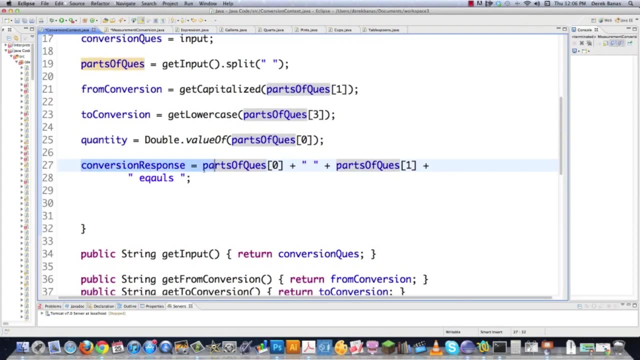 just gonna go question and get response which we created earlier, which is gonna be the beginnings of this. so let's just go over here. see, get response is right there. so conversion response. and where does conversion response come from up here? see conversion response, which is gonna spit out this guy right here. so if it's one, 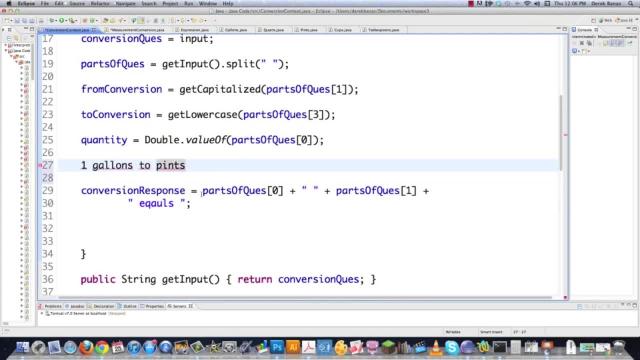 gallons, two pints. what's this gonna spit out? what's gonna spit out one, and then what's it gonna spit out? parts of question gallons, and then it's gonna say equals. and I need to spell equals. right, there we are. so that's what's gonna come. 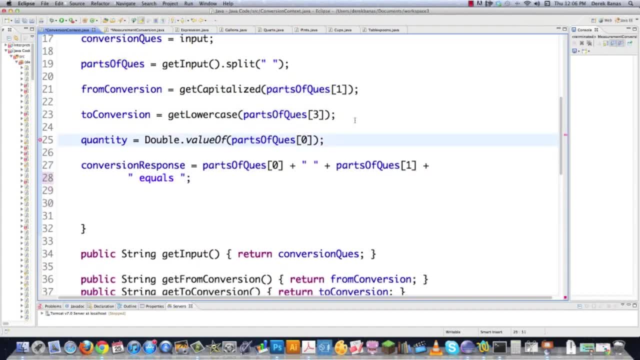 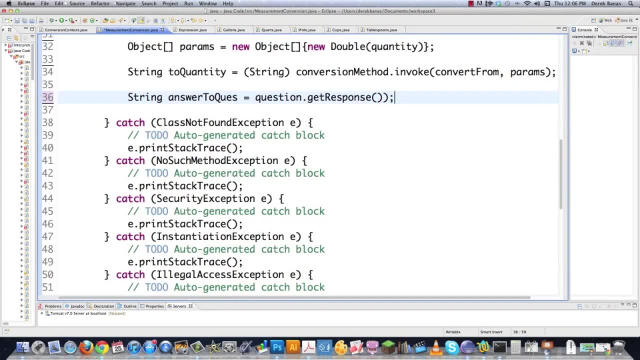 out and there it is. that's our going to be the beginning of our response to our answer. let's save that, jump back over into measurement. so that's what this guy is gonna do. so let's store that in our string. here is just go in here and go plus, and then I'm gonna go to quantity. is this guy? 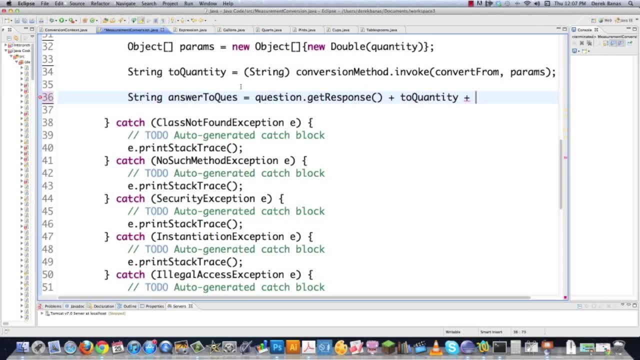 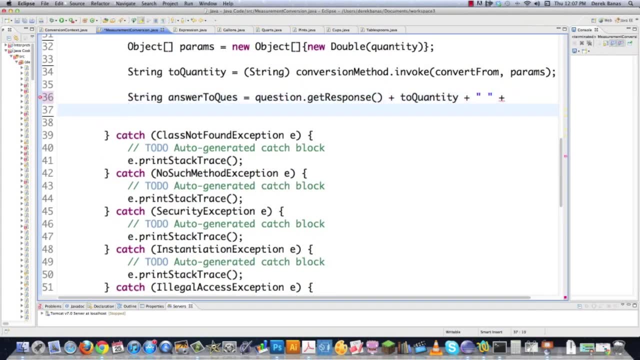 right here, it is the new converted. whatever you're converting into, this is going to be a number, and then we'll put a space in there and in another place and then we're going to define: what are we converting to? well, to conversion is what we're converting to. close that off, close that off and then we go, so that's. 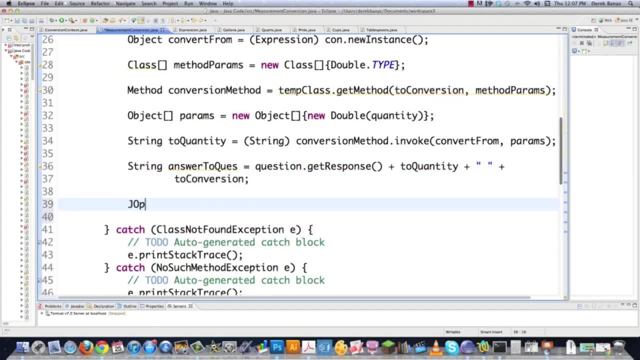 our answer that we're gonna be shooting out, and then all we need to do is shoot our answer out. so we'll go J option, pain show, message, dialogue- and we're just going to go null in this situation, and then the message we're going to provide is answer two questions. so let's paste that in there and then, after they click, okay, if we.